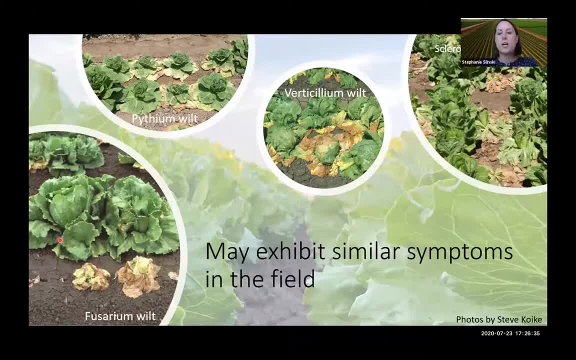 Complicating the situation. these diseases can occur in the same location. For example, in California growers are seeing Pythium and Fusarium wilt occurring in the same field. It's possible that without the Pythium infection, the Fusarium wilt would not become a problem. 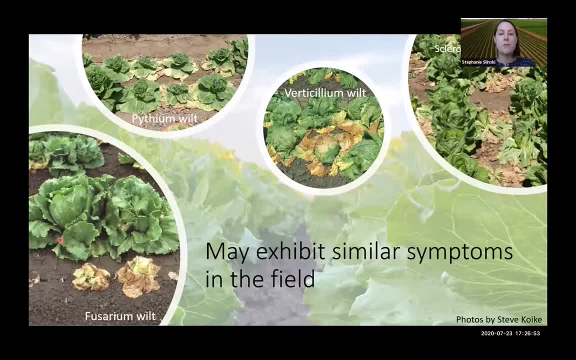 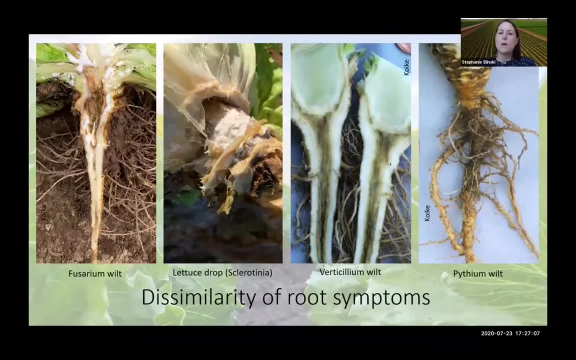 as Fusarium has been a resident of California soils for decades, It's often without causing significant crop loss. One way to differentiate the diseases is to examine the crown and the root system. These pathogens produce pretty distinct symptoms. You can see that Fusarium wilt and Verticillium wilt. those are both vascular pathogens and 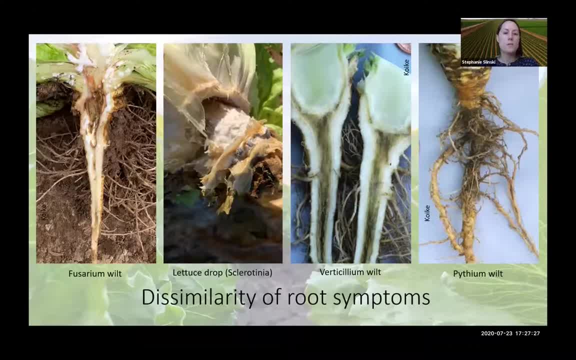 so you have to slice them apart. You can see that Fusarium wilt and Verticillium wilt. those are both vascular pathogens and so you have to slice them apart. You can also slice that root open to see those symptoms in the vascular system. 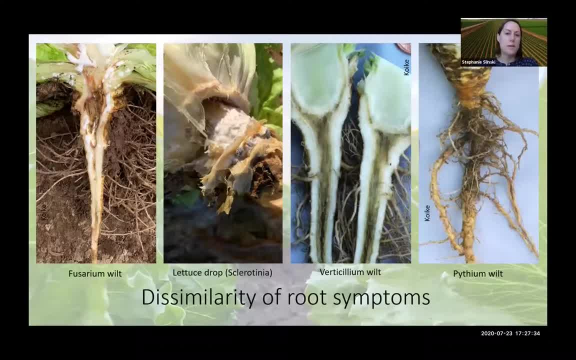 You can differentiate these pretty easily. The Fusarium wilt generally has the brownish or reddish symptoms where the Verticillium is more a bluish or blackish symptom. With lettuce drop you see the Sclerotinia in the crown. 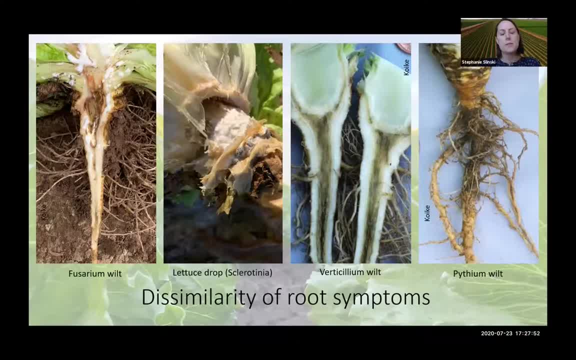 You also see some signs of the disease there with the Mycelium and Sclerotia. but that's distinct from fusarium and verticillium, because you have that rotting of the crown And then another example here is pythium wilt And that gets into those fibrous. 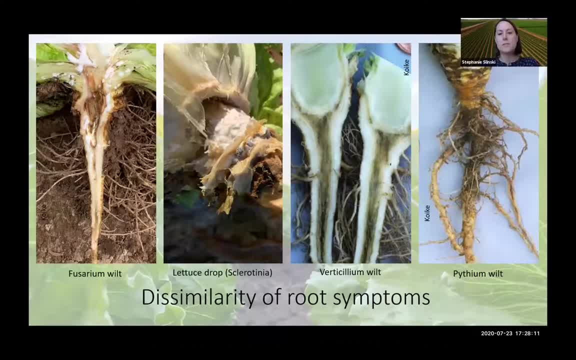 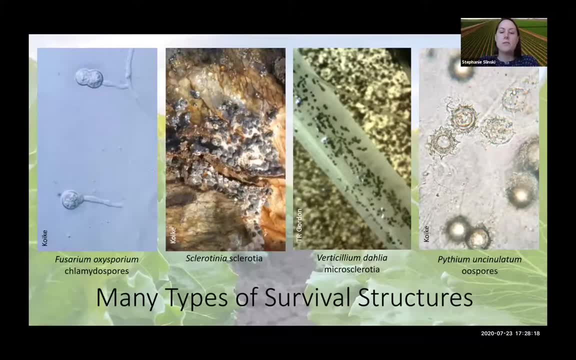 roots and rots the root from the outside. These pathogens also produce different survival structures. These are durable structures that can protect against desiccation, UV and other environmental stresses. Some examples are the chlamydospores of fusarium, sclerotia verticillium and sclerotinia oospores of 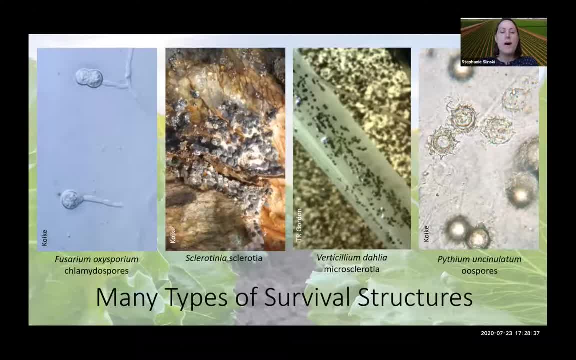 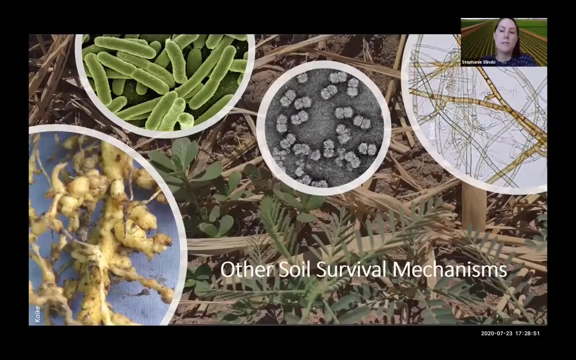 pythium. These pathogens can survive using these survival structures for years in the soil. And there's also other mechanisms of survival. Other mechanisms of survival, Other mechanisms are something like alternative hosts, like weeds or in crop debris. These act as a reservoir of these pathogens. Some of the pathogens like fusariums sclerotinia. 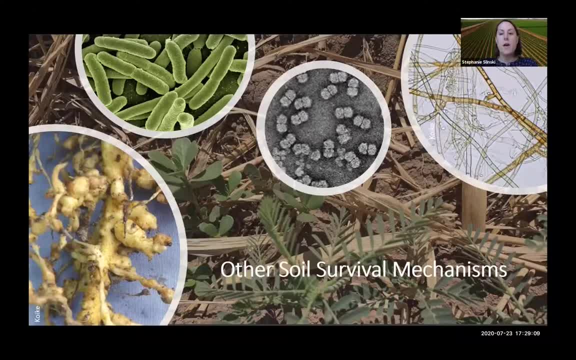 they will survive in these types of materials And there's also some pathogens that this is their primary survival mechanisms, like with Rhizoctonia, that's here that it primarily survives as mycelium in crop, debris or in other hosts, And also viruses can survive in weed species. 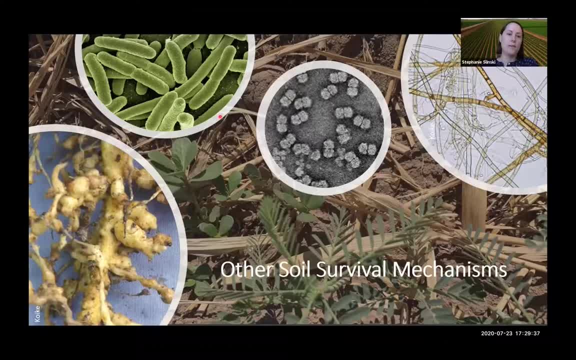 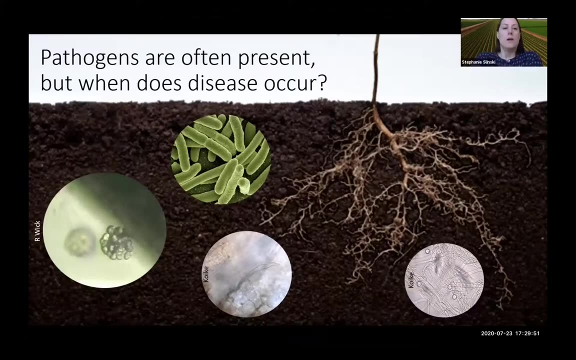 or in other vectors, Bacteria, and here's some root knot nematode, infected roots, So there's many mechanisms for surviving in the soil. If you sample the soil and analyze the microbes found in that sample, you might find many pathogens present. However, disease may not occur even if the presence of a highly susceptible, even in the presence of a highly susceptible plant. 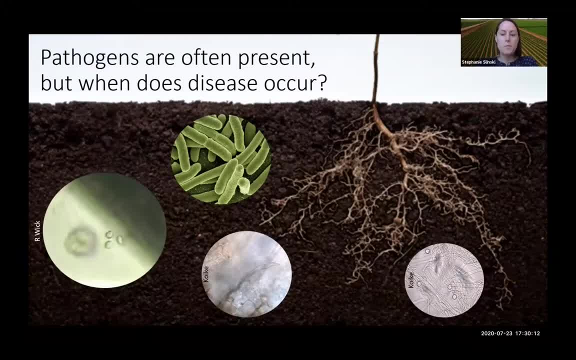 Here's a little video of pythium sporangium germinating. It releases these modal zoospores that are attracted to the sugars and the amino acids that are exuded by the plant. Here's a little video of pythium sporangium germinating. It releases these modal zoospores that are attracted to the sugars and the amino acids that are exuded by the plant. 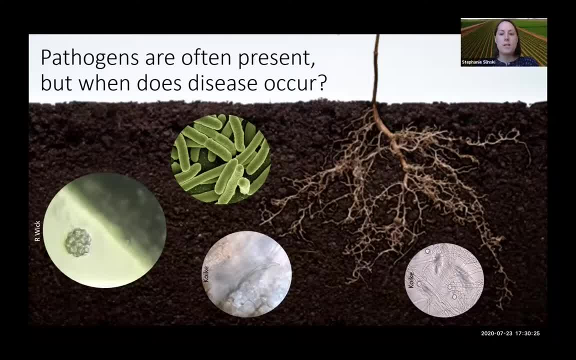 They swim towards the roots and lose their motility, germinate and infect the plants if nothing stops it, if it has the opportunity to reach those roots. Here's an unanswered question of when does disease occur? Pythium and simulatum has been found in Arizona soils for decades and it's been isolated from lettuce roots that did not show symptoms of a disease. 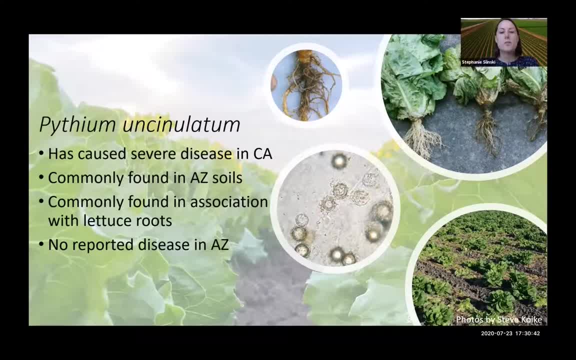 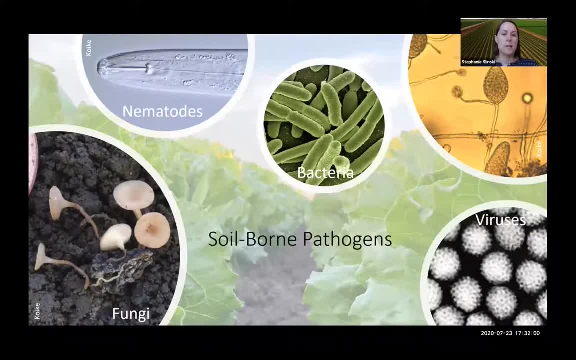 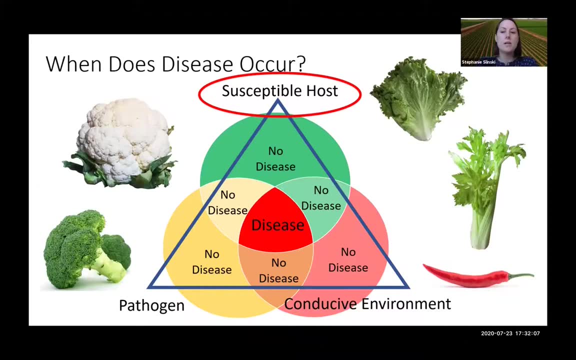 Pythium and simulatum has been found in Arizona soils for decades and it's been isolated from lettuce roots that did not show symptoms of a disease and this I give you some examples of this in previous slides. a susceptible host is another corner of the disease triangle. this could mean a host that 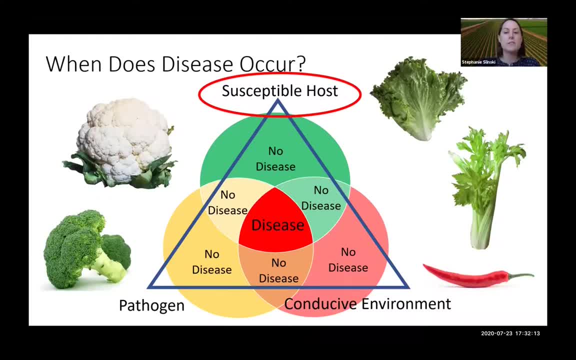 does not have a genetic, does not have any genetic resistance against the pathogen. this could mean that the hosts could not put energy towards defense. it could mean a host that was not primed to resist the pathogen attack. could mean a host that did not receive a pesticide treatment that prevents infection. it 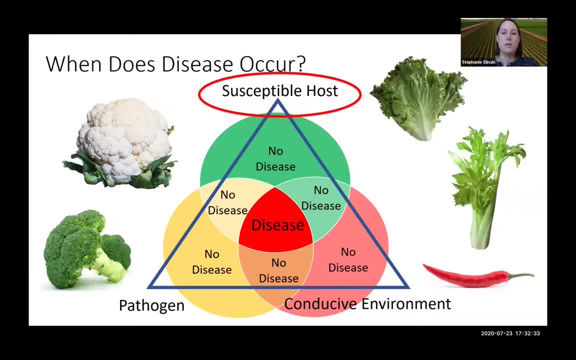 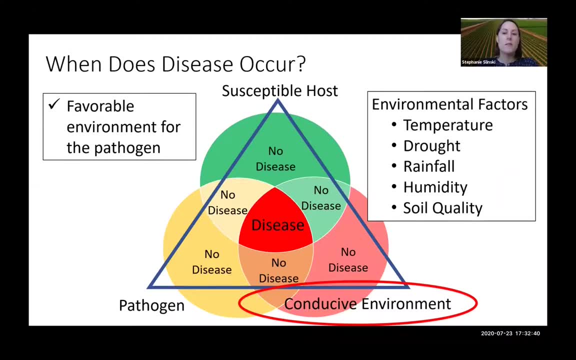 means the host is available for colonization, and a conducive environment is the final corner of the disease triangle. this is an environment that promotes disease by favoring the pathogen. this could be a climate such as temperature. an example of this is fusarium. molt of lettuce will develop in. 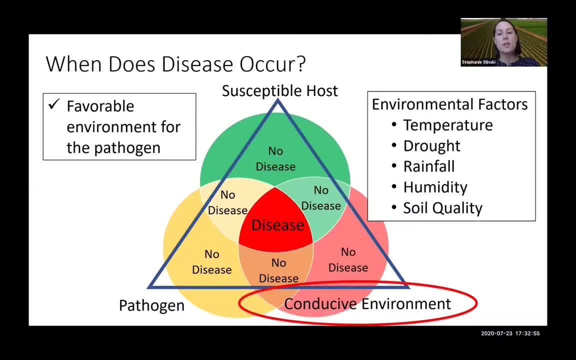 Yuma on lettuce planted in the desert early in mid-September when the temperatures are very high. The pathogen likes these warm soils. This is also a time of year that really promotes that plant stress in the lettuce, because the lettuce prefers to grow in much lower temperatures. So we might be seeing 90,, 100, 110 degree weather. 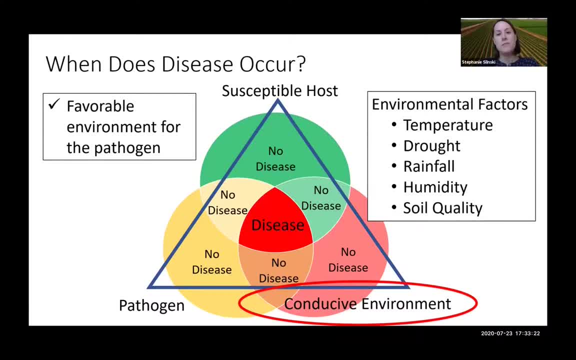 in September, while the lettuce wants to grow in 70 degree weather, So that makes the host more susceptible. Soil quality is another factor that could influence both the environment and the host susceptibility. Soil health is an important part of effective plant disease management. effective long-term disease management. 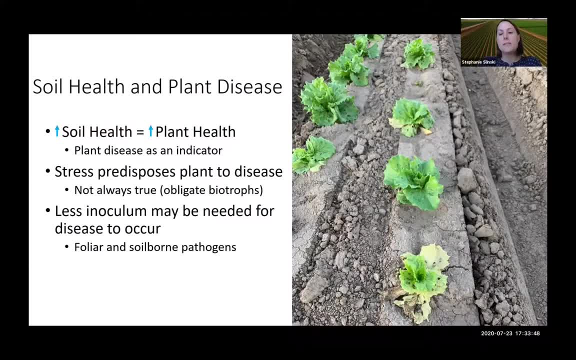 Soil health and plant disease go together. Often, we see disease as an indicator of problems with the soil. This can be caused by plant stress or could be caused by high inoculant levels in the soil. It's an indicator of a less diverse microbial community. 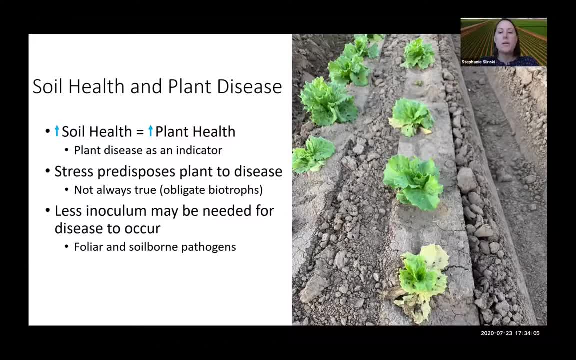 because an active and diverse microbial community will not support high populations of a single microorganisms And to add to that you also need to have a significant biomass of that microbial community. Plant stress does not always cause higher levels of disease. with some diseases, like downy mildews, Less disease may occur in. 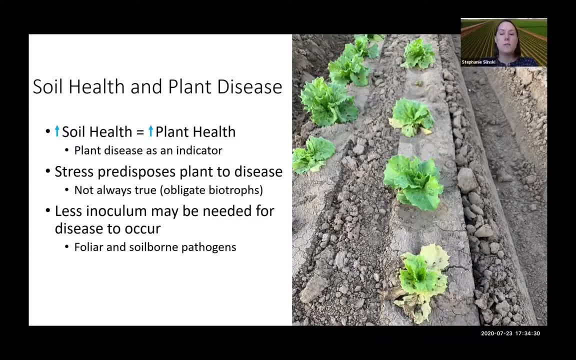 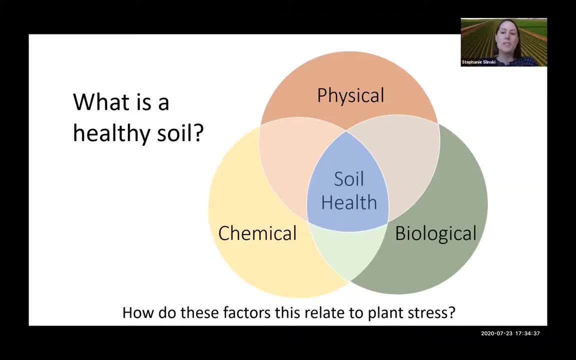 stress tissues, but I'm focusing on soil borne diseases here. I'm glad that I don't need to go into soil health, since that's been well covered in previous talks and I'm not an expert in this area. I do, however, want to remind you that there's three general 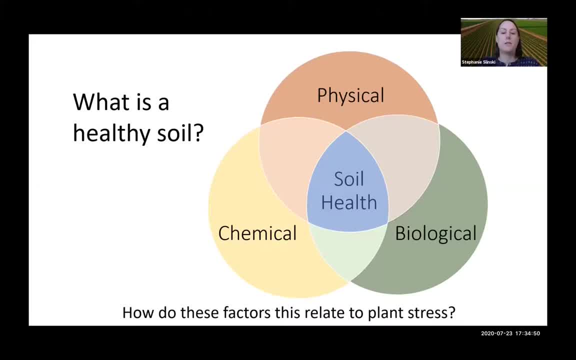 factors that are part of that, that are part of that that come together to form healthy soils. that's the physical, chemical and biological aspects of soil health. I want to bring these, remind you of these, so I can introduce to you some factors that contribute to plant stress. so here's some examples of those physical, chemical and biological. 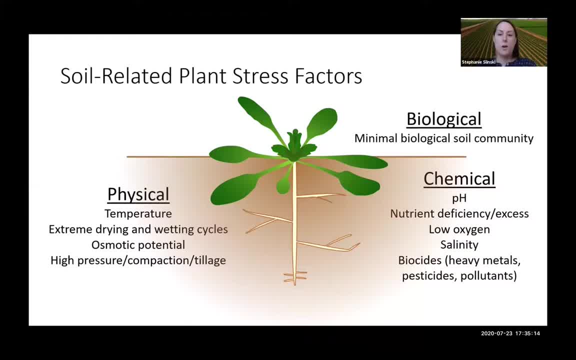 stressors. it's important to understand that those physical and chemical stressors will also have a negative effect on the biological aspect of soil health, so they they affect those soil microbes and the other biological elements to the soil. we'd like to have healthy soils for effective soil change. 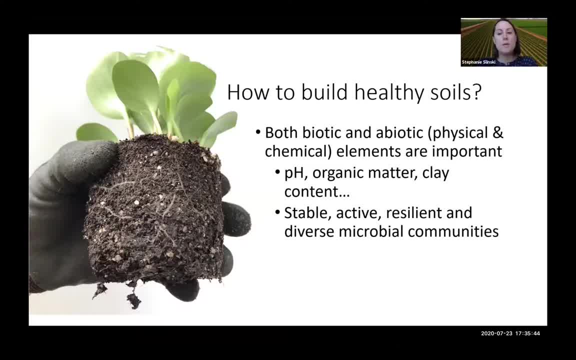 long-term soil-worn plant disease management. We want to have the physical and chemical factors to promote plant growth and reduce stress. We want a stable, active, resilient and diverse microbial community. Of course I mentioned there's other aspects of the biological community. 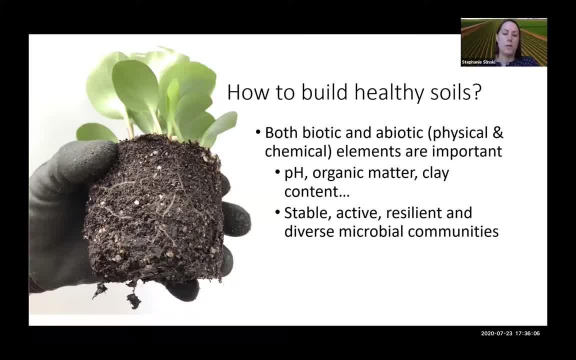 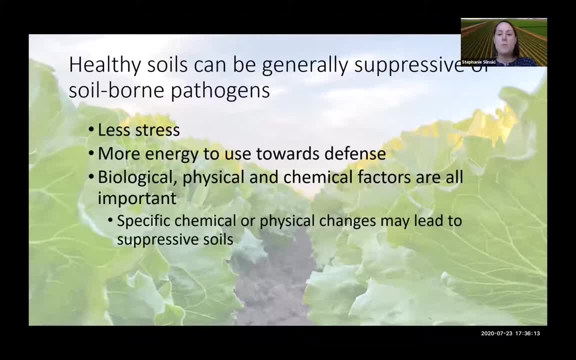 In the next slides I'm going to talk about the microbial communities. So you know that healthy soils reduce plant stress. Reduced stress also allows the plant to focus more energy on defense against pathogens. Physical and chemical factors are also important for suppressing pathogens separately from plant interactions. There are some studies that have 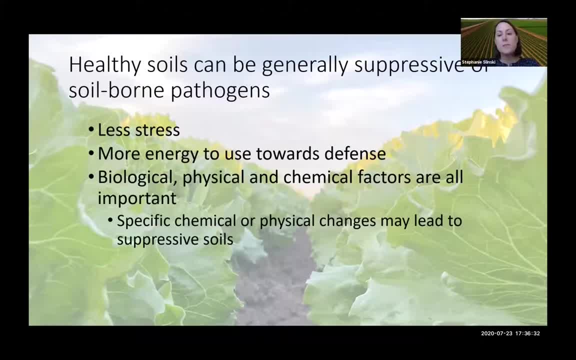 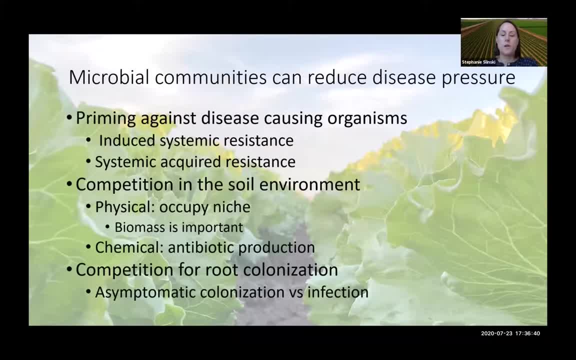 pathogen off you desk. pathogenization will help increase resistance and reduce presence. So that is going to be a numbers eight piece. Microbial communities in the soil can significantly reduce disease pressure. Some microbes can help build up the plant defenses by stimulating the plant to produce defense-related chemicals or 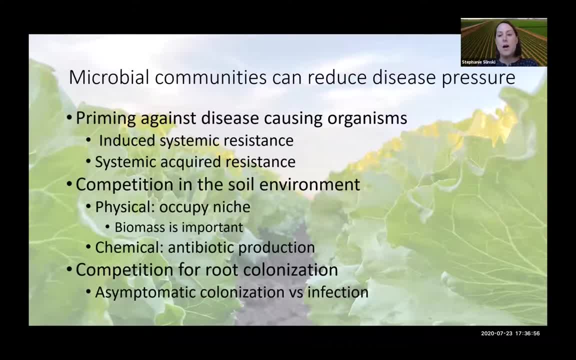 physical defenses against the pathogen, but competition in the soil environment is a much more general method to suppress disease. This could be by occupying the same niche as the plant pathogen, especially in the rhizosphere, which is that area around the roots influenced by the sugars and 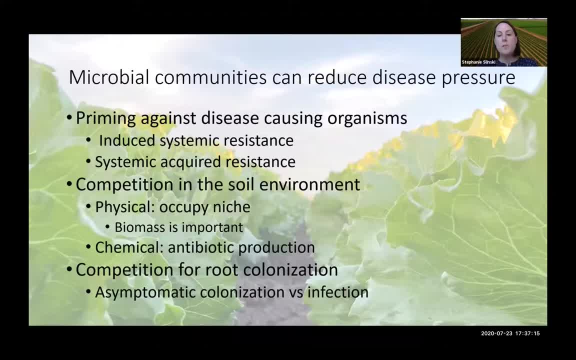 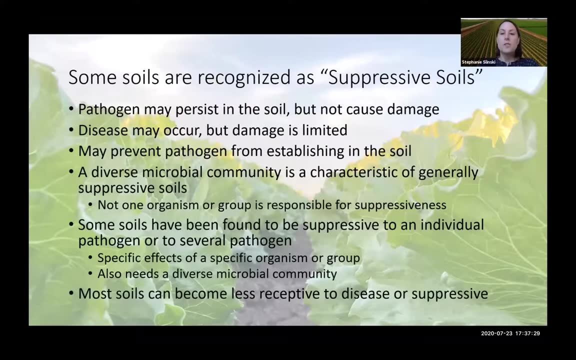 amino acids that are released by the roots. Some microbes will colonize the surface of the roots or will grow into the roots without causing disease. This is a very effective method of excluding pathogens from the root. There are soils that are recognized as suppressive soils. These are soils where the pathogen may. 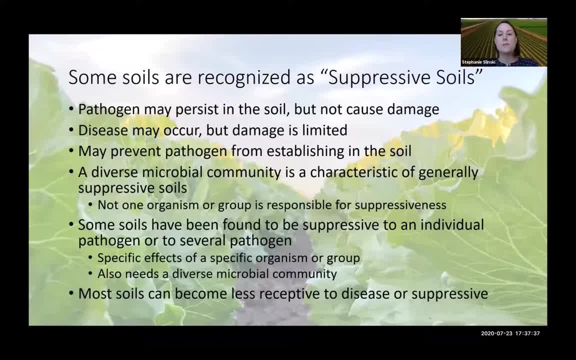 be in the soil but causes little to no disease. It is possible to have symptoms. Usually, the symptoms are a lot less severe than if the soils were not suppressive. The soils could help prevent pathogens from establishing in the soil. One of the characteristics of suppressive soils is that they have a. 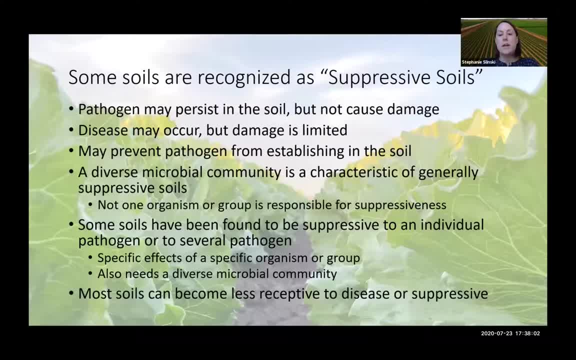 diverse microbial community, which is an indicator of soil health, Dr. Thank you, Dr. Usually, no one organism is responsible for that suppression. However, there are soils that are suppressive to specific pathogens. This is usually from the effect of a specific organism or group. 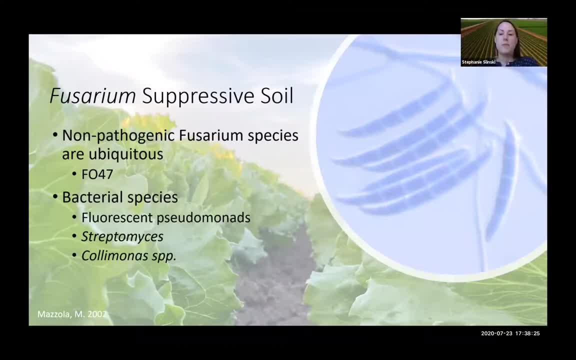 As an example, there are some soils that have been identified as suppressive to fusarium. There are several organisms that have been found to be responsible for this suppression. One organism that has been found to be effective is a non-pathogenic fusarium species. 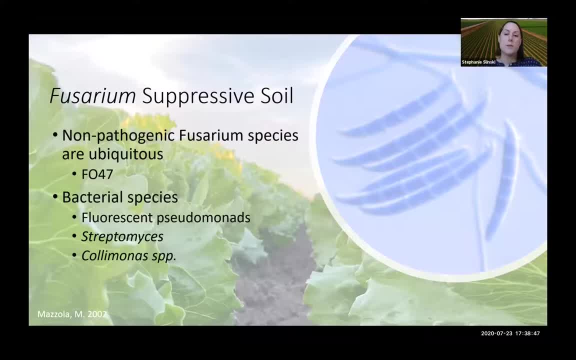 Fusarium oxysperm is ubiquitous in the soil. Many of the fusarium oxysperms that are found in the soil are not pathogenic on any plant species. These can out-compete pathogenic fusariums. Fusarium oxysperm is a type of species that is not 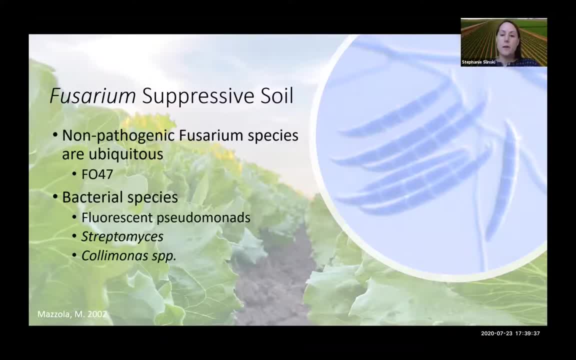 verticillium, verticillium dahliae, which is a common. it causes verticillium wilt, And this FO47 has also been found to be more effective when combined with other organisms, like specific species of pseudomonads, And there are other bacterial species that can also help. 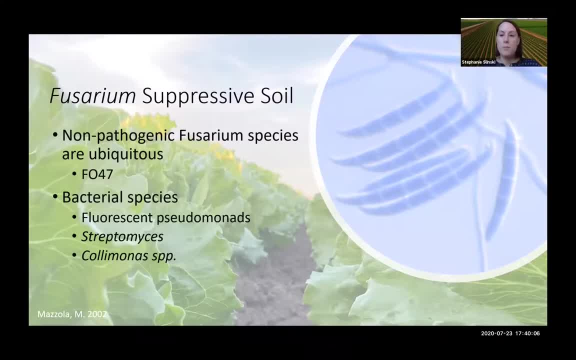 compete in the soil environment And it's often because they produce chemicals that will suppress pathogens, like antibiotics. So streptomyces make streptomycin, So there's different chemicals that are produced by these bacterial species in the soil. Unfortunately, FO47, there's no products. 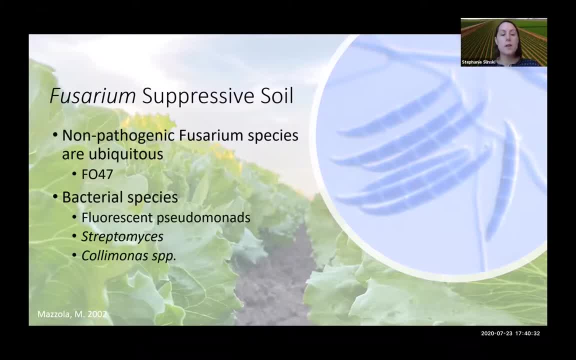 that are made. There were two products from Europe That were made with FO47, but they're not available, So it doesn't seem like even though this research is ongoing. I saw some research papers from this year that report on studies with FO47. It doesn't seem like there's much of a move towards developing a product. 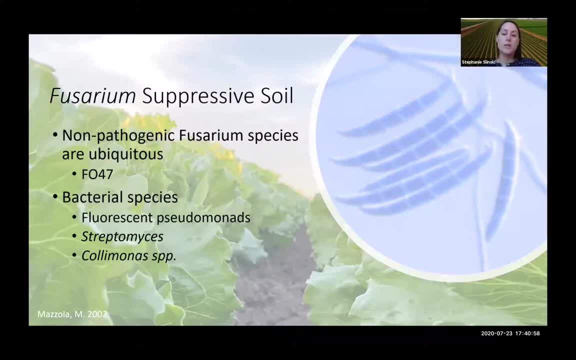 But it's good that research is continuing And there's other organisms that have been found to be effective against the bacteria that are responsible for this, So one single cell that has been identified as a very, very important organism. as far as what we're interested in is Fusarium, There's a colomonus isolate that was isolated by Johan Laveaux's lab from UC Davis that was shown to suppress Fusarium wilt of tomato. And these are studies that are pretty early on And so they are not being performed at field scale at this moment. but there are opportunities to develop products that could help develop suppressive soils or less diseases in the soil. 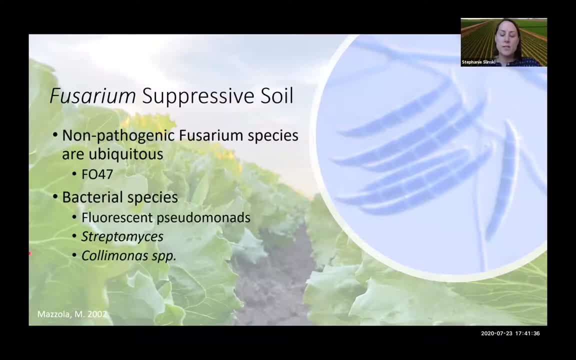 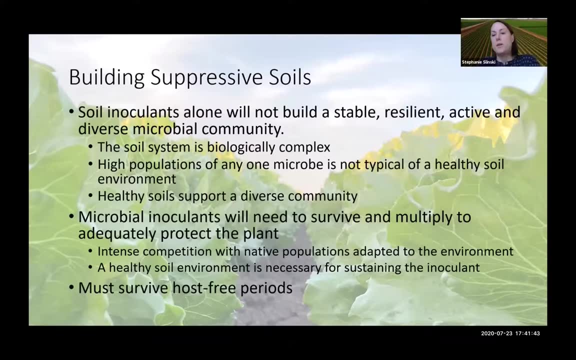 receptive soils, but a healthy soil is the starting point to all of this. When you decide to start developing suppressive soils, you may decide to use a soil inoculant. There are many inoculants on the market right now, but the inoculates alone won't build a stable 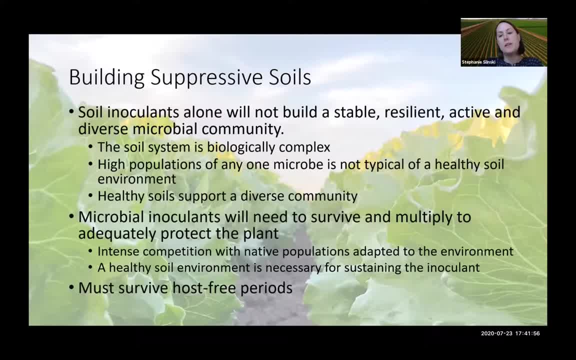 active, resilient and diverse microbial community because, as you know, the soil system is very complex, The microbial community is complex and it's not possible to create a formulation with the level of diversity that the natural soil environment has. and formulations need to be. 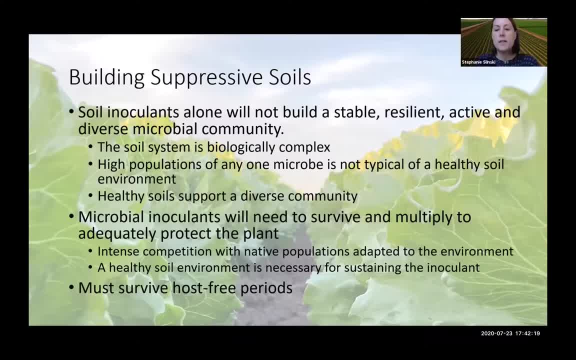 adapted to your environment, and the soils need to sustain the microbe and the formulation over long periods of time, including those host-free periods. But, as you understand from the previous slides, the microbe is a complex soil. The microbe is a complex soil. The microbe is a. 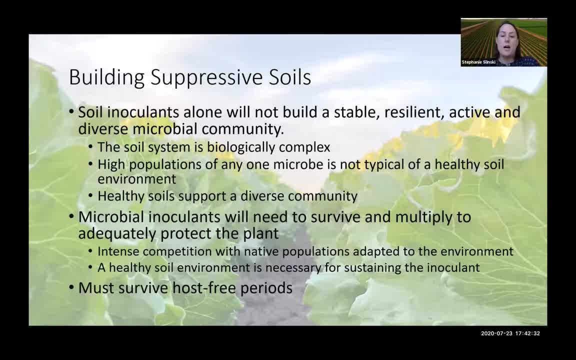 previous slide. there's a role for inoculants that can provide, if they can provide, the appropriate competitive microorganisms, and there can be a role for some of these products along with other methods to build soil health and support the native microbial populations. 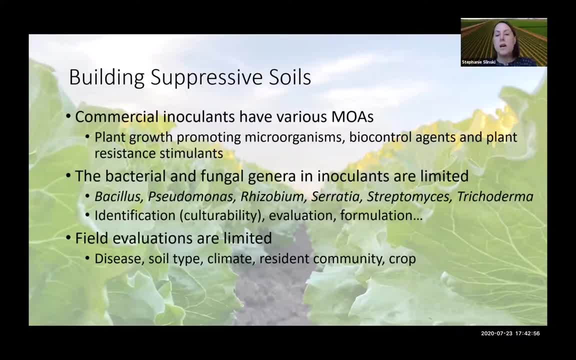 Commercial inoculants are labeled as having various modes of action. I discussed some of these modes of action in previous slides. These inoculants usually contain microbes from a limited group of genera, and this is because these are groups that have been identified. 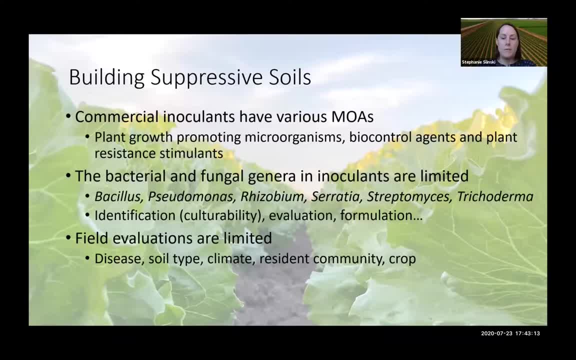 which means they can be grown in a lab or grown in a fermenter. They can be. they've been evaluated for specific modes of action. They can be formulated into a product so they have a shelf life, so they can actually be used in agriculture. 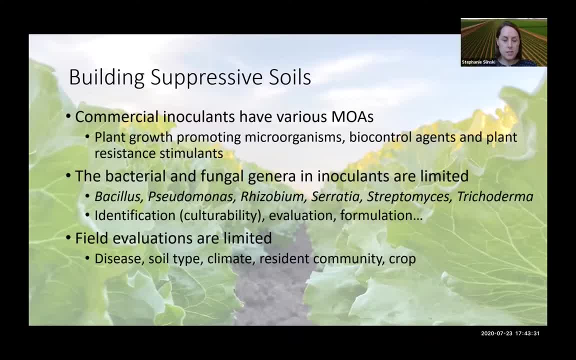 The genera that I listed are just maybe half of the common genera that are found in a lot of these products. It's difficult and expensive to evaluate products on multiple crops and growing regions, so efficacy data may not be extensive for your specific growing conditions in your crop, So you should carefully consider any product you decide to add to your soils. 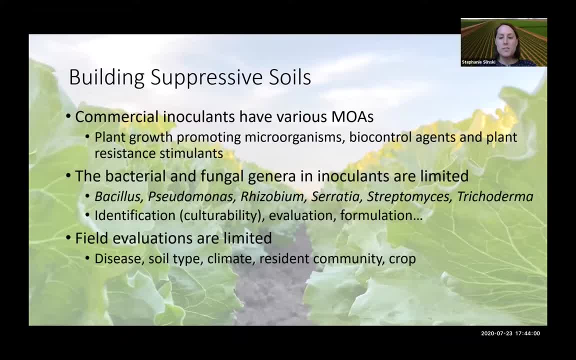 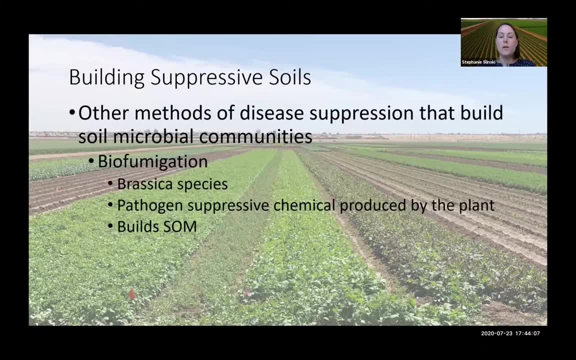 Consider your goals For your soil and use products and conditions that can sustain the microbial populations. There are some other methods to suppress disease and build soil microbial communities, including biofumigation. Biofumigation is the use of a brassica green manure that releases isothiocyanates. 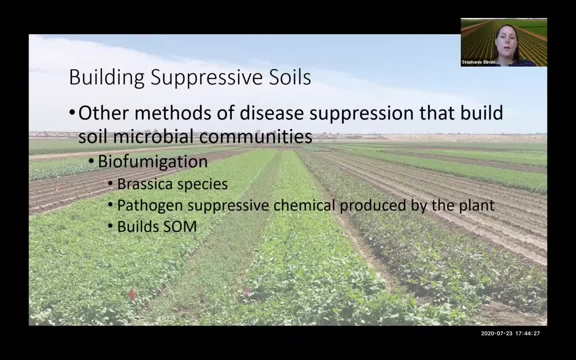 when the, when the crop, when the debris is incorporated into the soil and irrigated. This is a chemical similar to the active agent of the fumigant metam sodium, And the addition of the green manure helps to build soil organic matter. 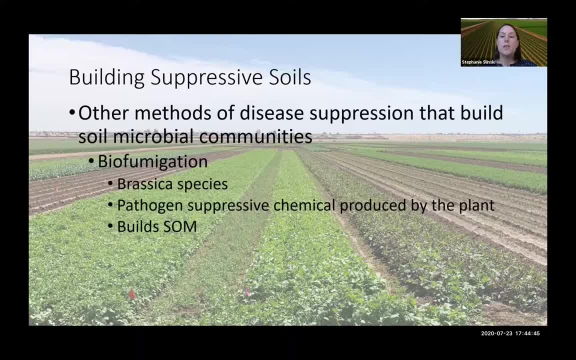 and build the microbial biomass in the soil. The most consistent success with this method is against nematodes, And this may be because nematode suppression does not rely on a completely organic material. So it may be that the nematode suppression does not rely on a completely organic material. 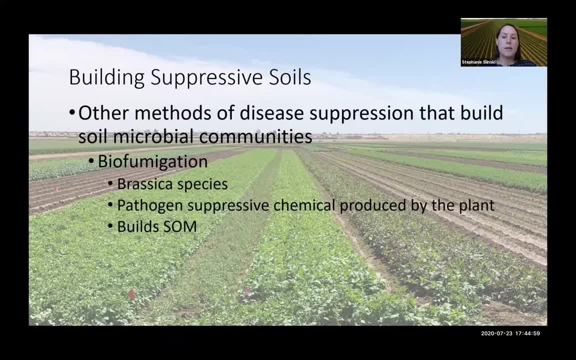 So it may be that the nematode suppression does not rely on a completely organic material- Thehigh levels of isothiocyanate- And there are other chemicals in the green manure that contribute to the suppression along with the isothiocyanate. 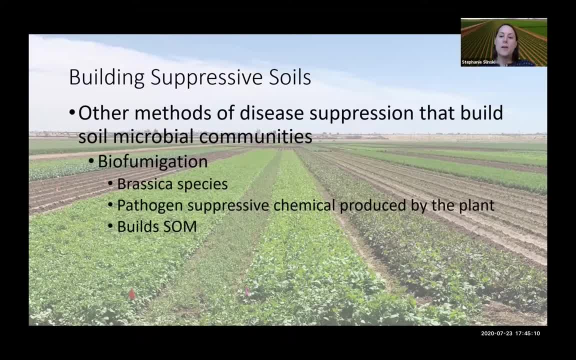 Biot veteran has been used to suppress many pests and pathogen groups, including nematodes, weeds, insects, fungi- Oh my seeds- and bacteria. but with midst success. timing is really important, both for when you have the highest level of the chemical and the mass has increased quickly. 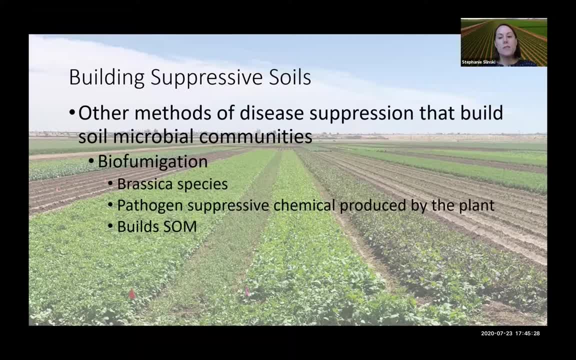 Titan, which can stimulate Хорошо in the plant and when the target is most susceptible. so you really have to time those, so they occur at the same time. and the method of incorporation is really important. you have to pulverize that plant material, and immediately. 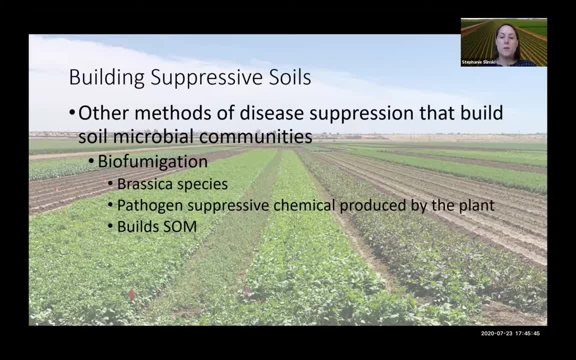 irrigate the soil. conditions have to be managed to maximize the production of these chemicals and also to minimize the volatilization of the chemical. it's a promising method of suppressing pathogens, but there's not yet consistent efficacy under field conditions. this is something that i've done a little bit of work with recently. 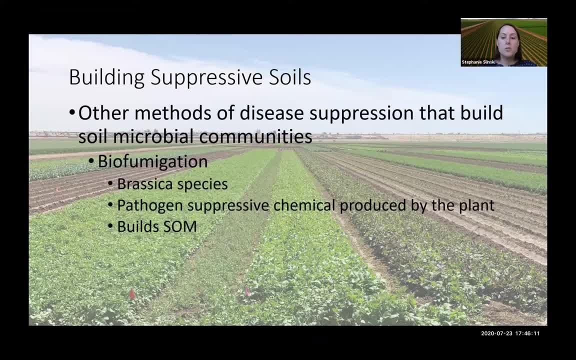 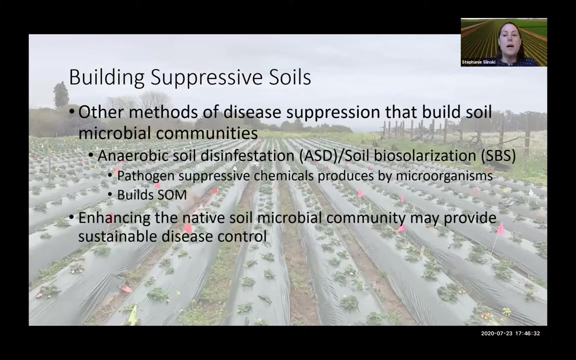 and also alex, who, from the university of arizona and tucson, has been doing some work. the background of this slide is some of some mustard that we planted this spring and we did a a pilot study to look at suppression of fusarium wealth of lettuce. another method of suppressing pathogens is by 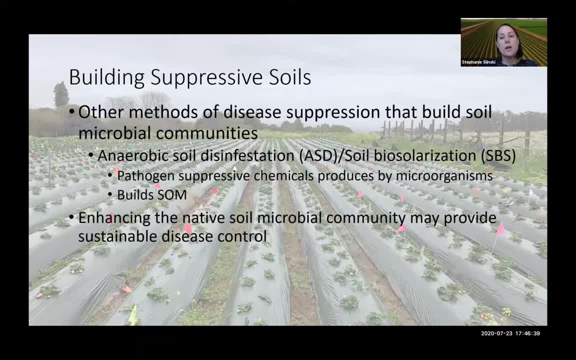 solar soil biosolarization or anaerobic soil disinfestation. the difference between these two methods is only that biosolarization is conducted during periods of high heat, which we have lots of in arizona, whereas anaerobic soil disinfestation- soil disinfestation- does not have the heat to get that that solarization effect. um, asd and sbs are. 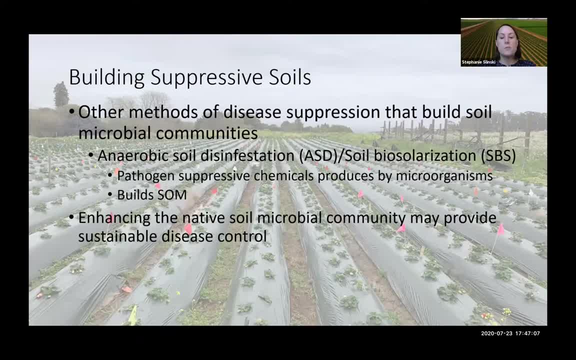 um, like i just said, they're similar to biosolar, is to to solarization, but um a carbon source is applied at a rate of four to nine tons per acre and the soil remains saturated for the duration of the treatment we put. you put this plastic on top, you saturate the soil, you have the carbon in. 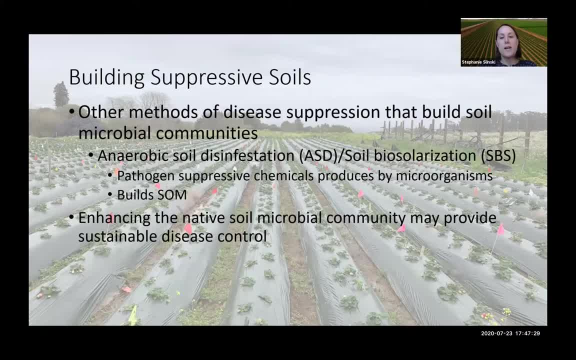 the soil and that induces anaerobic bacterial growth. it's hypothesized that the anaerobic bacteria produce chemicals that are antagonistic to the pathogens, but the mechanism may also be through antagonism, through niche competition um the. this method may suppress pathogens longer than solarization alone, by more effectively reducing the pathogen populations. 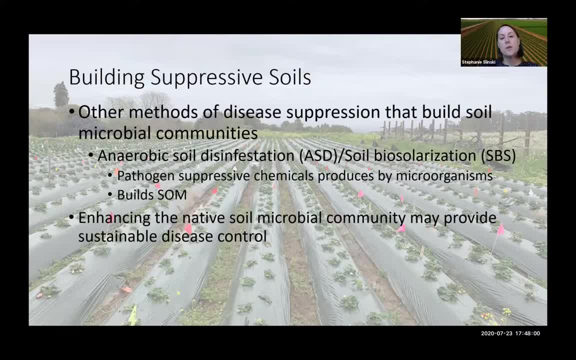 but it also might be because, with the addition of the soil, organic matter and the stimulation of the microbial populations, you're maintaining suppression of the pathogen, the pathogens, for longer than solarization. um, solarization can have a detrimental effect on microbial populations because you're just heating up that soil. you're killing a lot of. 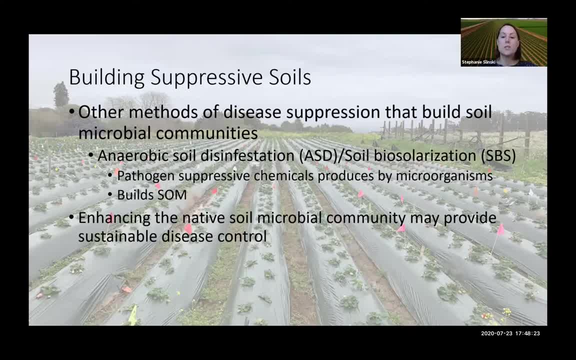 strong microbes in there, um, so it's hard to say what the effects are, but it's not a lot of inflammation and by the time you get away with it- those microbes in the soil- it's similar to fumigation. um. anaerobic soil disinfestation is currently being used in california to treat more.